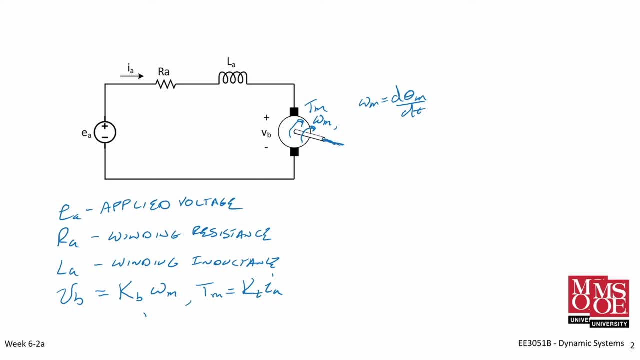 And that came from Lenz's law of force. Typically, the motor is going to be attached to some mechanical load And that mechanical load will have a rotational inertia- J sub L- And there may be rotational friction on this mechanical load. And I'll show it as a dashpot. 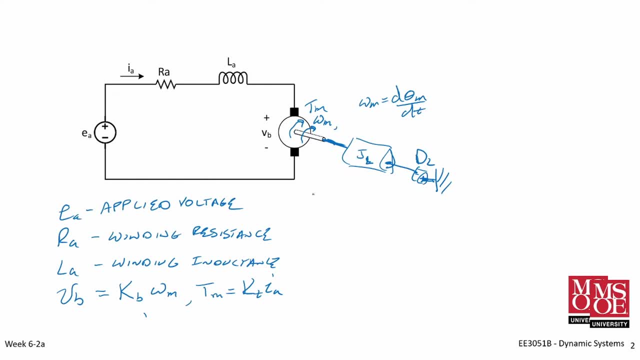 D sub L: The motor itself. the armature of the motor is going to have its rotational mass J sub A And will also have some friction in the motor, which I label as D sub A. Therefore, the total motor rotational inertia that the electric motor experienced J sub M is due to its armature plus the applied load rotational inertia. 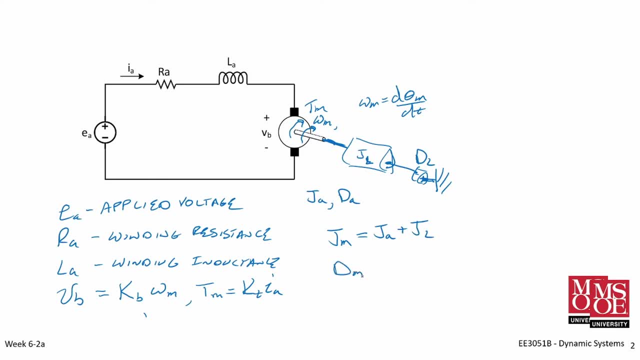 Likewise, the total frictional coefficient for the motor is due to the friction in the armature as well as any friction on the load. We can now derive an electrical equation for the motor, And then we're going to derive the mechanical equations, And these two sets of equations will allow us to obtain the transfer function for the DC motor. 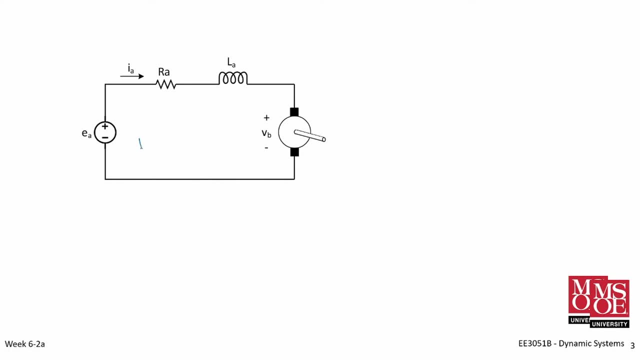 Let's obtain the electrical equations for our motor. We can do KVL around this loop And we see that Ea minus the voltage drop across the winding resistance, Minus the voltage drop across the inductance, And recall the voltage drop across an inductor is VL, is equal to LDI DT. 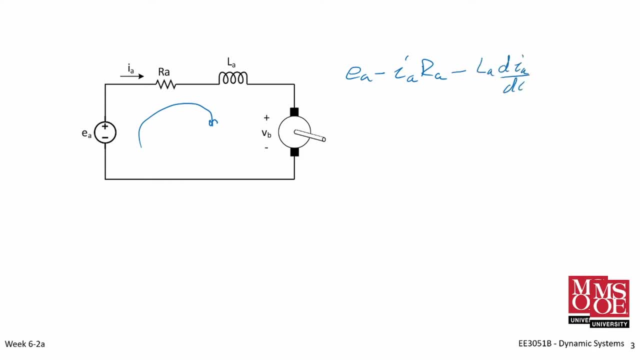 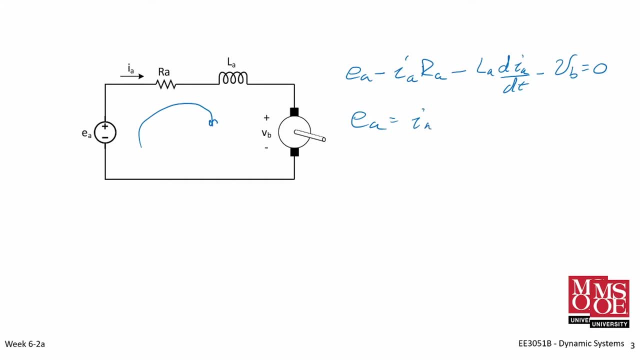 I'm going to rearrange this equation And we have: Ea is equal to Ia times Ra minus La times DiDT Plus, I mean plus plus VB. We can now do the Laplace transform And we obtain Ea s is equal to Ia times Allah. 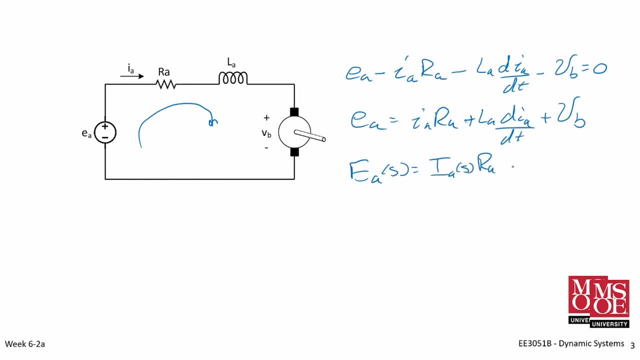 IA as a function of S, RA plus SLA, times IA of S plus VB of S, But note that the torque is related to the current through the following equations: I can do the Laplace transform of both sides of that equation to obtain: 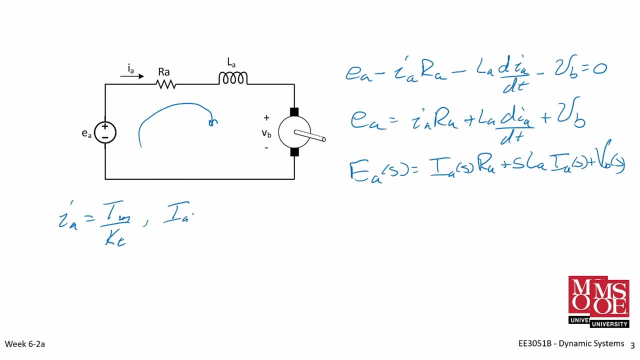 an equation for the Laplace transform of the current IA of S, And that is equal to the Laplace transform of the torque divided by the torque constant K sub T. And likewise the back EMF is equal to the torque constant K sub T. 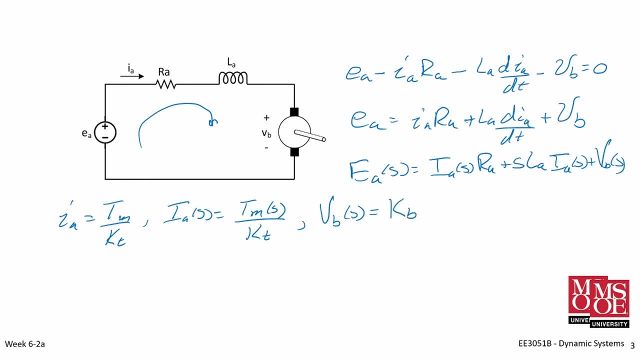 And likewise the back EMF is equal to the torque constant K sub T, And likewise the back EMF is equal to the motor constant KB times the Laplace transform of the angular velocity, which I'll write in form of the angular displacement. 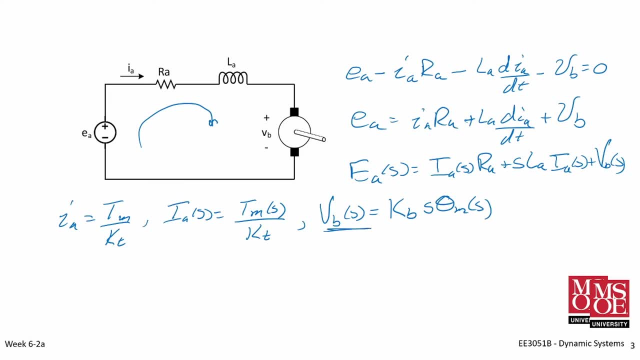 We can now substitute these two equations into our equation and we obtain: EA of S is equal to TM of S times RA, RA over KT plus TM of S times SLA over KT plus KB, S, theta M of S. Here's our equation for the electrical portion in terms of the angular displacement. 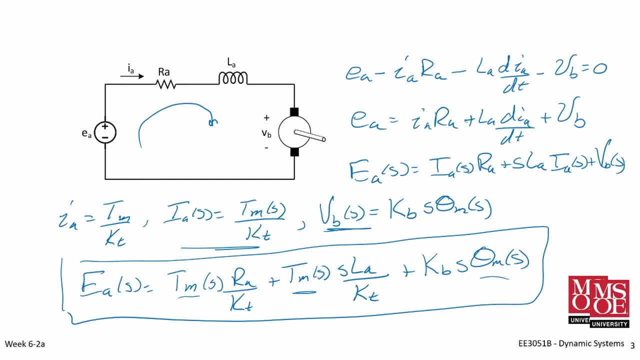 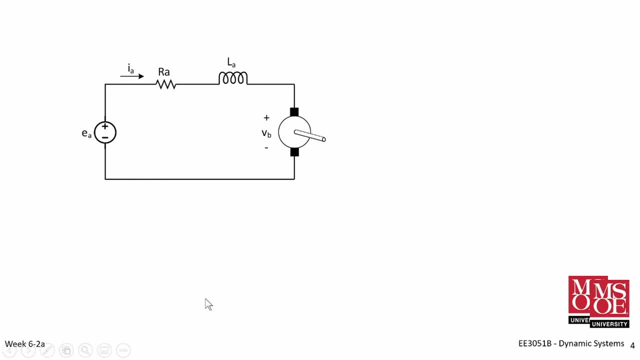 and the torque that the motor applies. We can resolve this equation by looking at the mechanical equations. So now let's look at the mechanical equations and recall that the total inertial mass that the motor experiences, J sub M, is equal to JA plus JL. 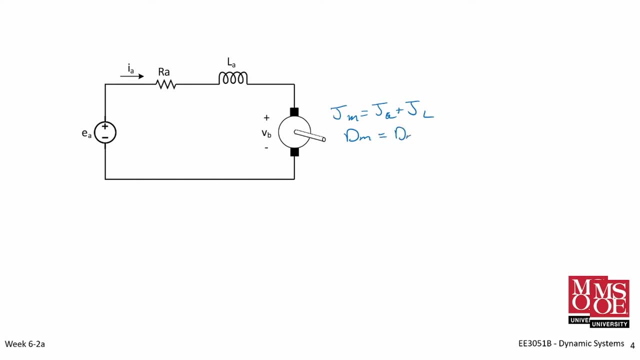 and DM is equal to DA plus DL and the motor is going to apply a torque T sub M to that total load the motor experiences. We can do a free body diagram on this rotor and I'm going to do our free body diagram directly in the Laplace domain. 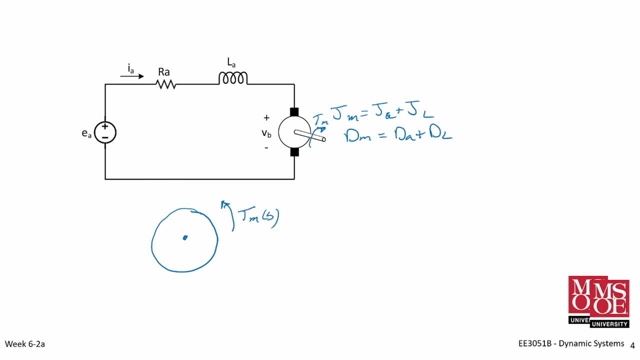 We have an applied torque- TM of S. we have a counter torque due to the rotational mass- JM S- squared- theta M of S- and we have a counter torque due to the friction- DM S- theta M of S. This results in the following equation: 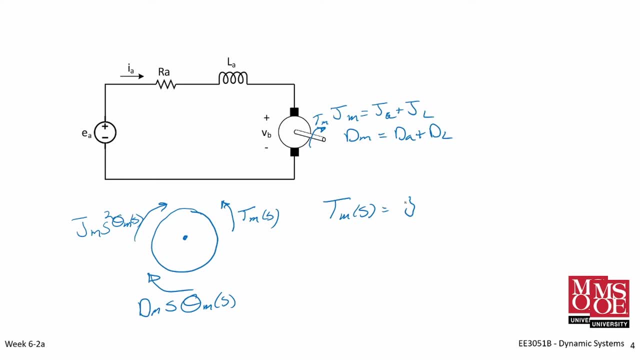 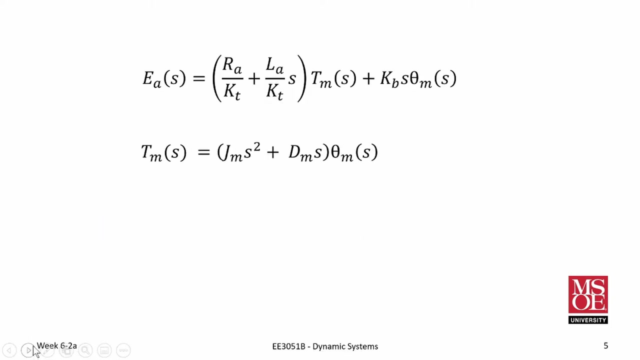 The torque is equal to JM S squared plus DM S, all times theta M of S. We now have an equation that relates the torque to the angular displacement, which we can use in our electrical equation. and here I've tidied up the electrical equation and we're going to now substitute our torque equation into the electrical equation and that 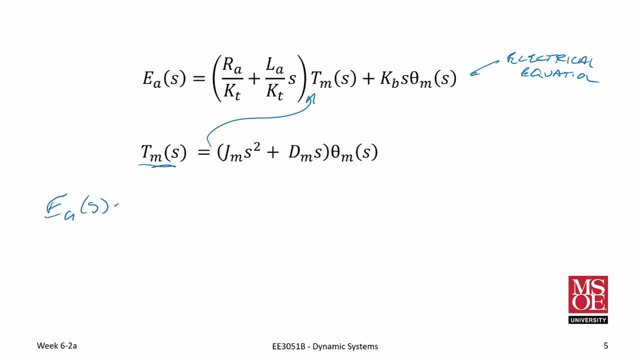 provides us with ea is equal to r a over k t plus l a over k t s times j m s squared plus d m s, all times. theta m of s plus k b s. theta m of s. we can factor out a theta m from from the right hand side of this equation. 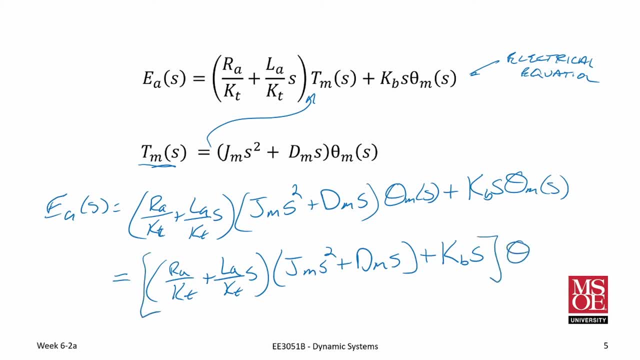 and we can then substitute our torque equation into the electrical equation. one of the things you may notice is we have a third order system. it is common practice with the motor models to ignore the inductance l a, because l a is much, much smaller than r a and therefore its term and effect on the startup. 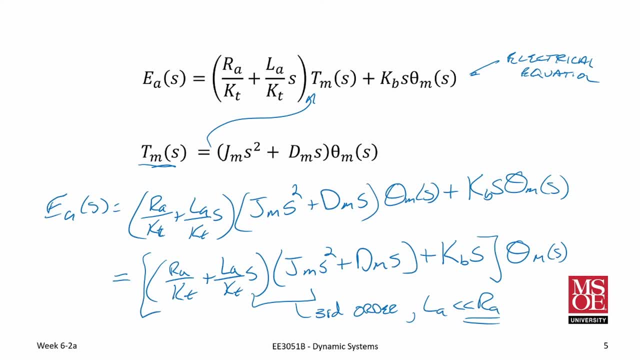 properties of of the dc motor are somewhat negligible. they're there but they're not that important. and the the transient effect it causes is so quickly, it goes away very fast, and so oftentimes we ignore this term and we we let l a equal to zero. so let's look at that situation. 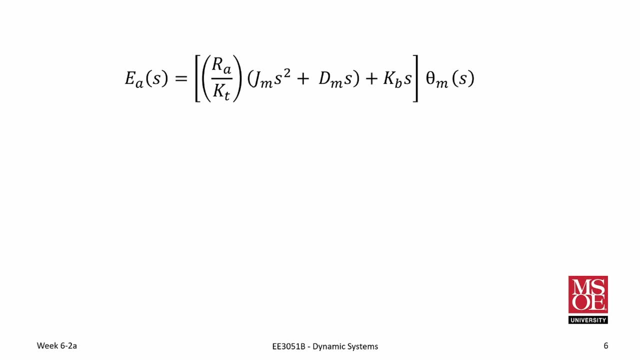 where l? a equals zero. here we show the equation. that's tidied up and we have l a set equal to zero. we can rearrange it a little bit more. let's combine terms of s in this equation and we see we have r a j m over k t s squared plus. 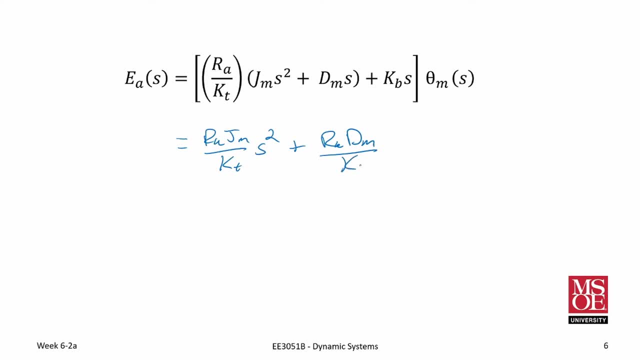 r a d m over k t s plus k b s, all times th. Theta M of S or RAJM over KT S, squared plus RADM over KT plus KB times S, And now we are set to write this in terms of Theta M over EA is equal to 1 over. let me take an S out of this equation. 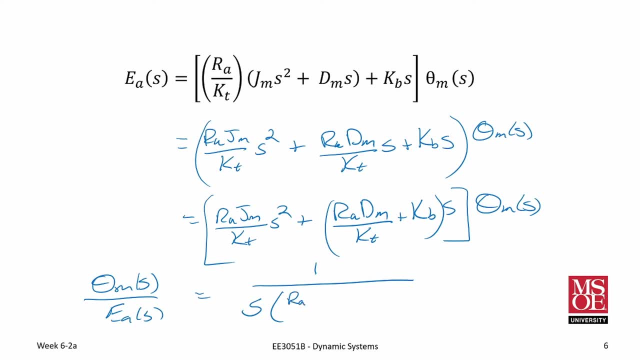 S times RAJM over KTS plus S plus RADM over KT plus KB. Now, as you know, we typically want to clear this leading coefficient. Therefore, we're going to multiply both top and bottom of this equation by KT over RA times JM. 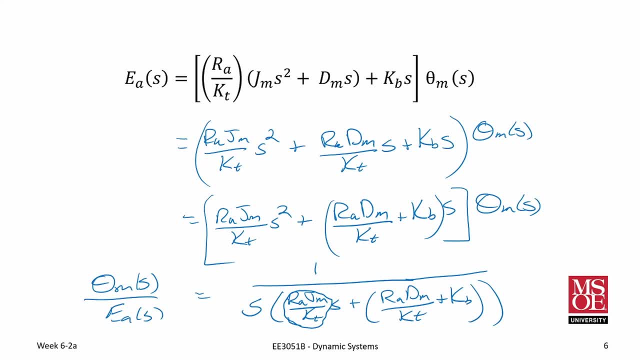 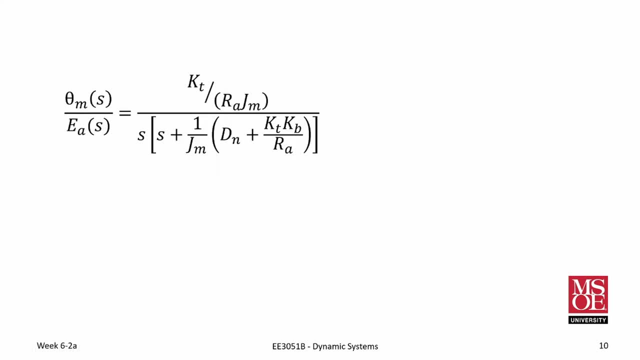 Again, we're going to multiply by KT over RA times JM, And this is the equation we obtain when we do that. Here, we see that we've cleared that coefficient out And we're left with this term. This has the form of A over S times S, plus A. 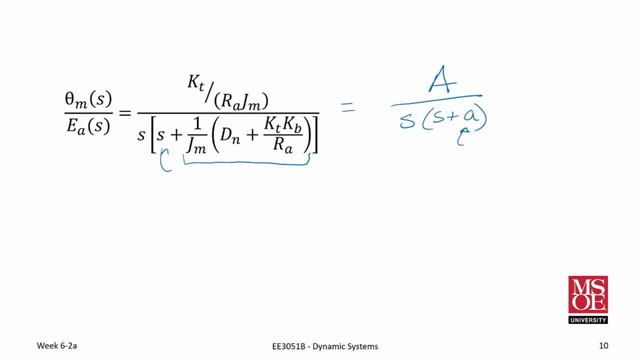 And this should look very familiar. This little A acts like our time constant, Where A is equal to 1 over tau for a first order system. therefore, that should be an m right there. therefore, our tau for our dc motor is equal to one over this term.